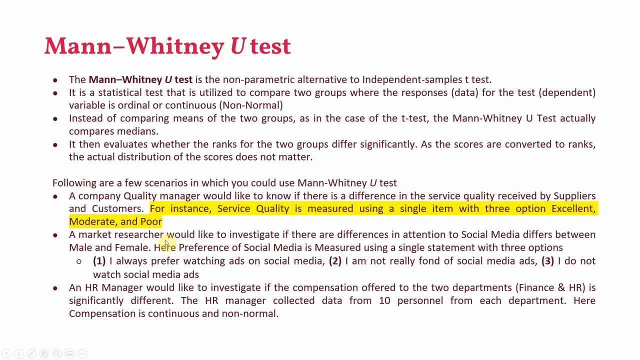 like to investigate if there are differences in both situation, also Inside-out αν cocoabad, Fear of the might, Mitages experiences 對 쪽 seekers higher, more漸展 tính attention to social media, and whether these differences are significant between male and female. here the preference for social media is measured. 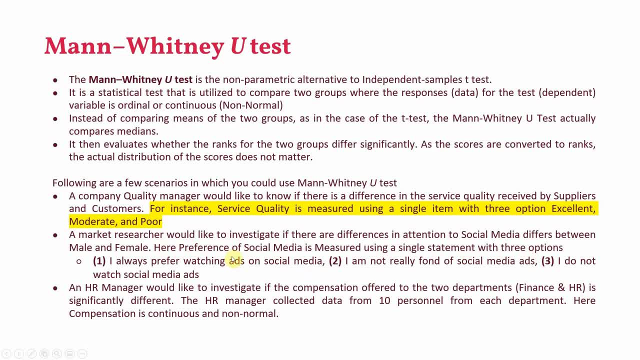 using a single statement that has three options, and these options are on ordinal scale. so in both of these first two examples your data is in ordinal scale. here there are three options: excellent, moderate and poor. and in the next example there are also three options. one always prefer watching ads on social 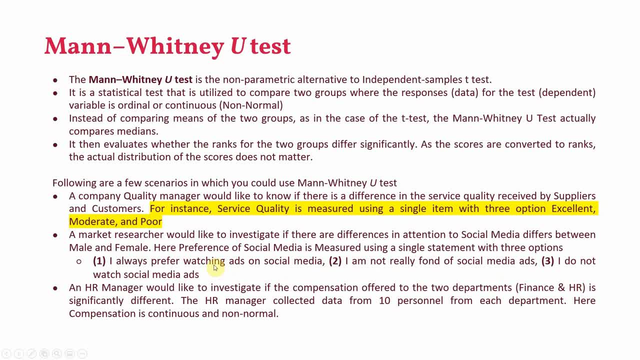 media. I'm not really fond of social media ads. I do not watch social media ads. however, the last example: an HR manager would like to investigate if the compensation offered to the two departments, finance and HR, is significantly different. the HR manager collected data from ten personnel form. 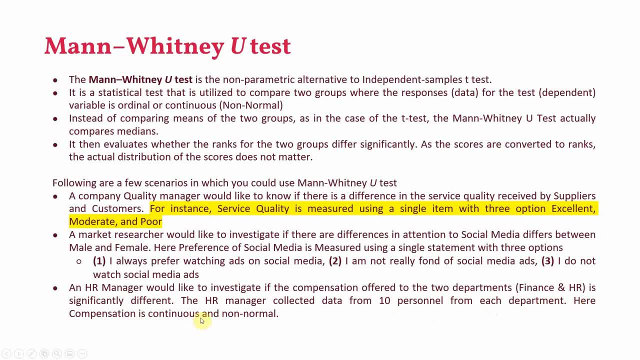 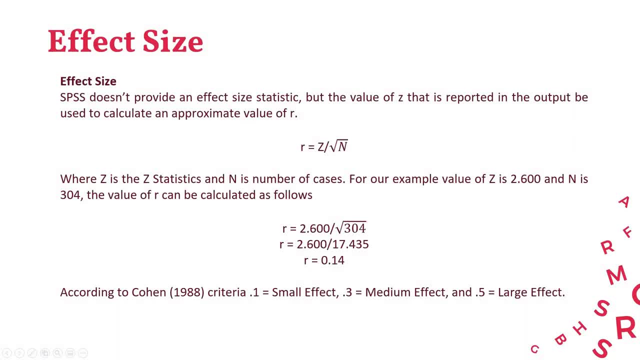 from each department. Here the compensation is continuous but non-normal. So we can go for Mann-Whitney u-test. So if there are groups, there must be a difference, and that difference must have effect size. So SPSS does not provide us with effect size, but we can calculate it. 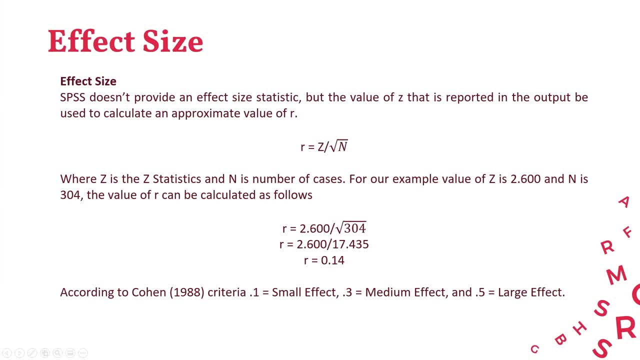 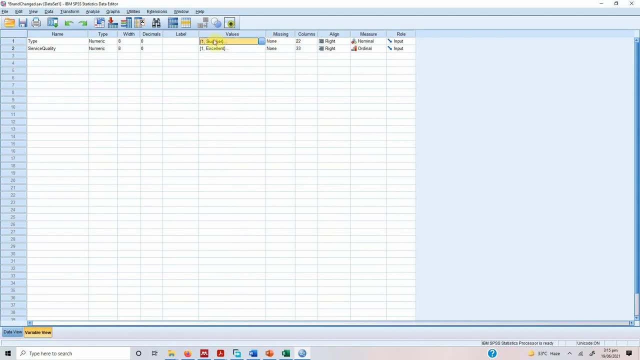 using this formula, which we will do at the end of this session. So here is our example data, The type- this is our categorical variable- supplier or customer, and each supplier and customer have given their rating of the service quality. Now, since this is on ordinal scale, 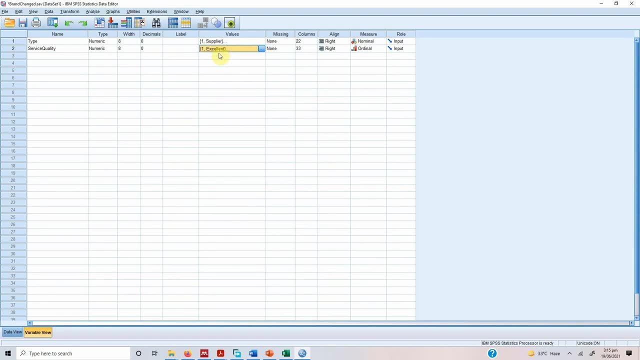 the test variable is on ordinal scale and we are interested in identifying whether this service quality rating differs between supplier and customer or not. So in order to do this, we will go to analyze. So we have two different test variables: non parametric test, legacy dialogs and two 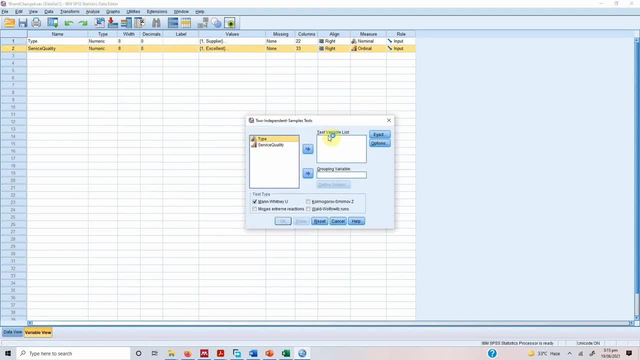 independent samples. Why two independent samples? Because we have got two groups: supplier and customer. So we click on this. What is your test variable? We are interested in checking the differences in service quality, So the test variable will go here because we are. 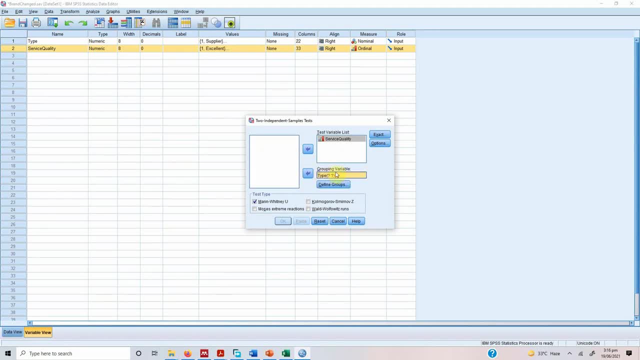 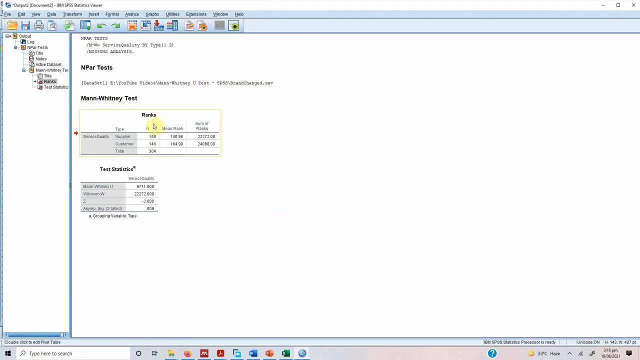 interested in service quality differences: supplier. so this will go here. this is our categorical variable: define groups: one for supplier, two for customer. press continue and press ok for results. now here are our results. so the sample size is suppliers. there are 158 suppliers. this is just a sample data. 146 customers. the mean rank: well, it's low for supplier. 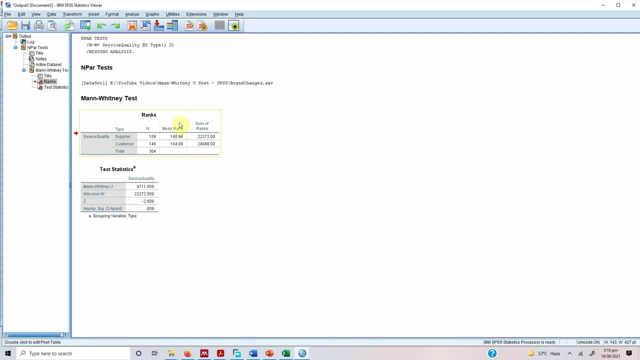 high for customer. so are there significant differences in the mean rank? well, the results show that this significance value. here, point zero zero nine is less than point zero five. so this shows that there is a significant difference in service quality as perceived by the supplier and customers. so the service quality offered to the suppliers and customers there is a 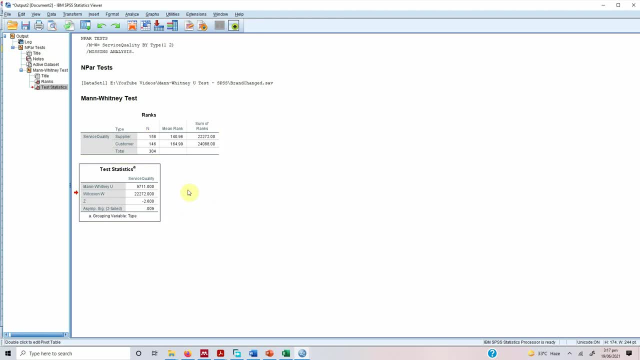 significant difference. so, yes, there is a significant difference. you is this difference moderate, small, moderate or large? and this is done through effect size. so how do we calculate the effect size? we need a Z statistics. we do not need to worry about the sign, because we are interested in. 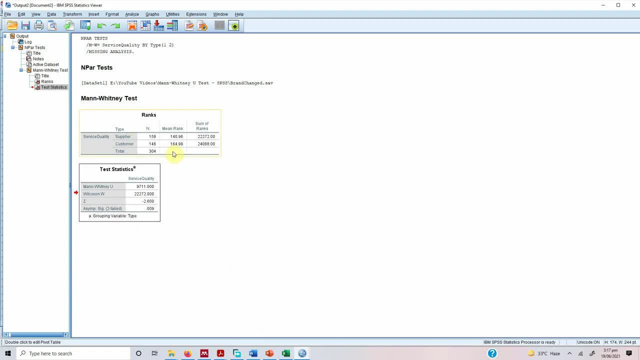 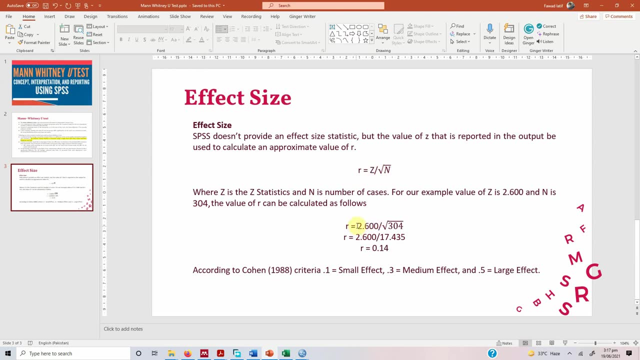 the effect size, not the direction of effect. so two point six, zero zero. so what we'll do is Z and N. Z is two point six zero zero. the total sample size is three zero four. so we will take the square root of three zero four. that will come down to seventeen point four three. 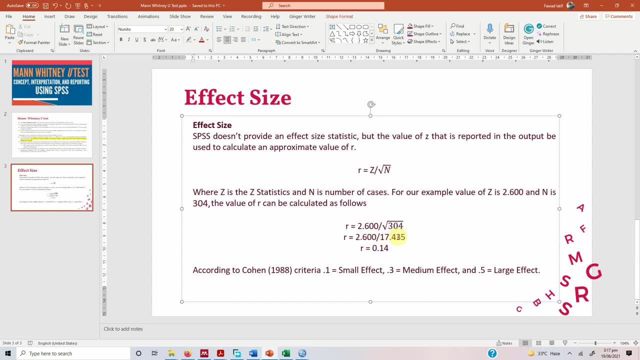 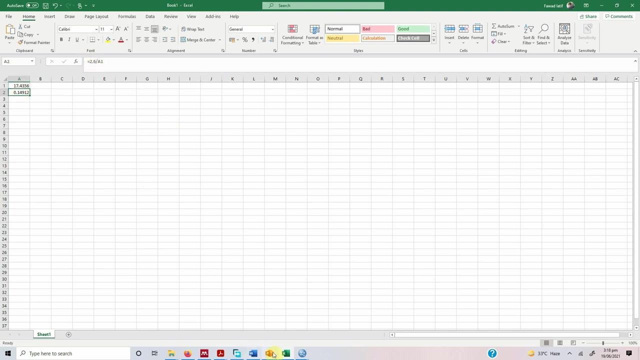 five. so two point six, zero, zero, which is your Z value, divided by seventeen. point four, three, five will give us point one, four, and this shows that there is a small effect. the difference is not that big between the customers and the suppliers, so let me be sure about it. well, yes, the difference is point one, four. 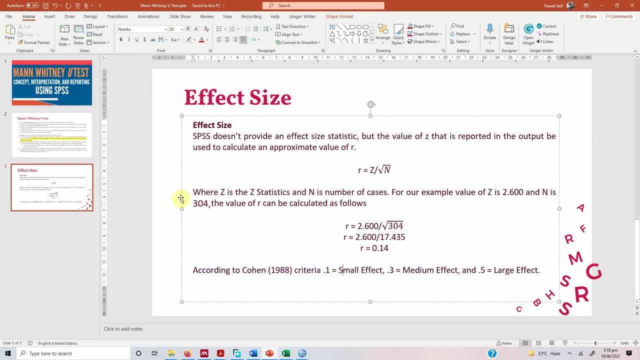 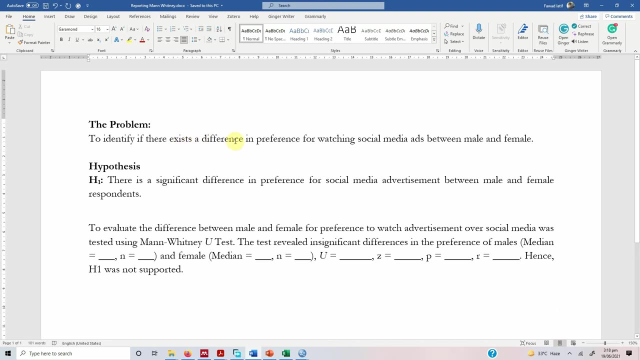 so the effect size is small. now how do you report? man Whitney, you test, so the difference in service quality is small between suppliers and customers. so how do you report these results? so let's change the problem a bit to identify if there exists a difference in service quality. 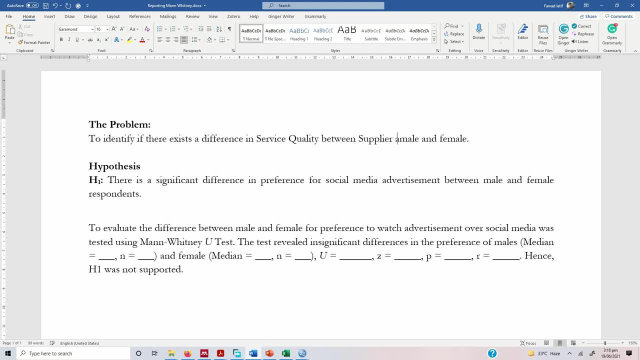 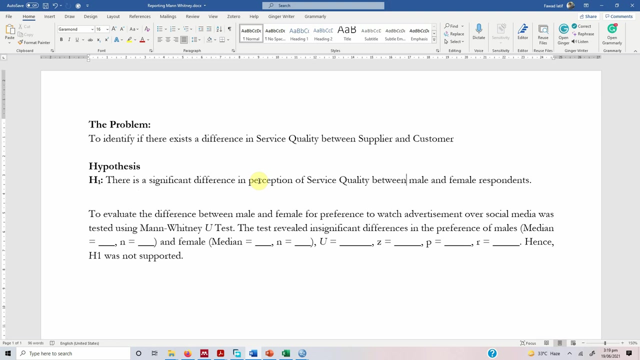 between supplier and customer. so here is our problem. so there, like we translate this problem into a hypothesis, there is a significant difference in, let's say, perception of service quality between supplier and customer. now how do you report these results to evaluate the difference between supplier and customer for service quality, which is our test variable, and 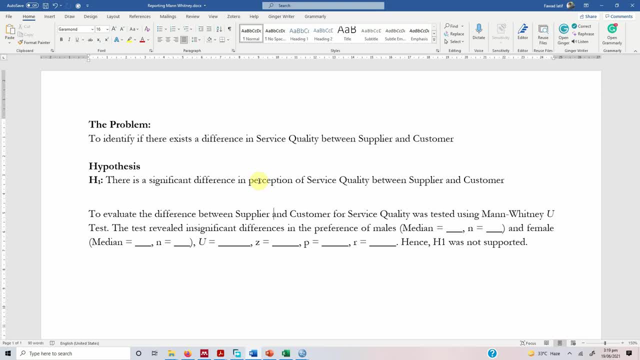 this was tested using man Whitney you test- let's correct the English a bit- man Whitney you test was utilized. the test revealed- and in this case it was- significant differences in service quality, of service quality perception of suppliers and customers. so what are the median values? let's see. so we need the median values, how to get them go to. 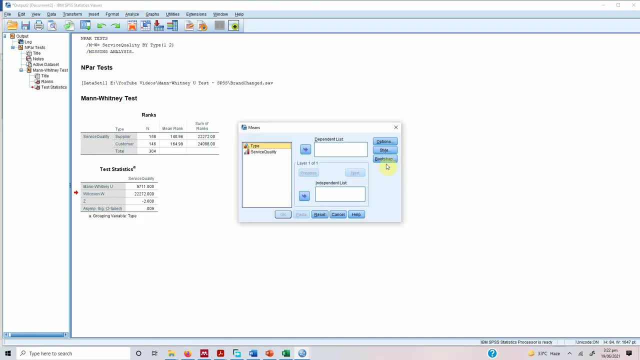 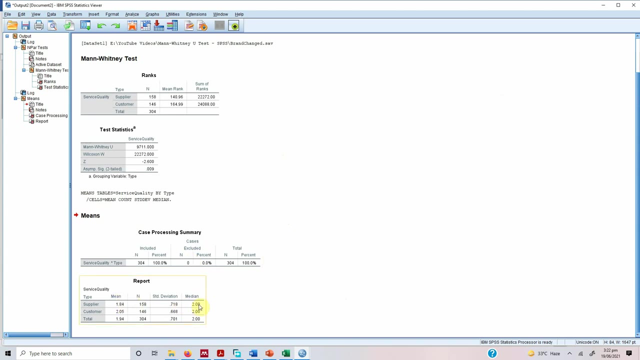 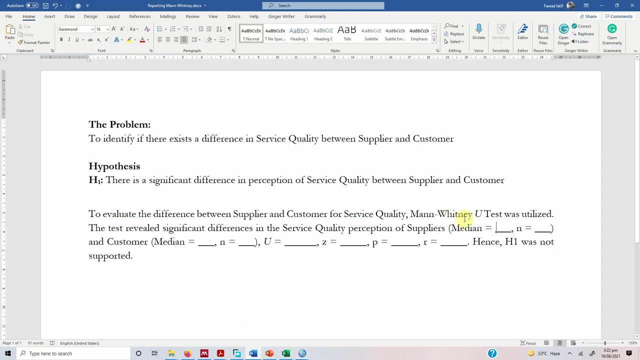 analyze, compare, means means. so the dependent variable is service quality. the independent is this type: go to options, select the median here. put it here: press, continue, press, ok, and the median is for both of them it's two, two. so the median where you is to two. so let's say the median value is to the end for suppliers. 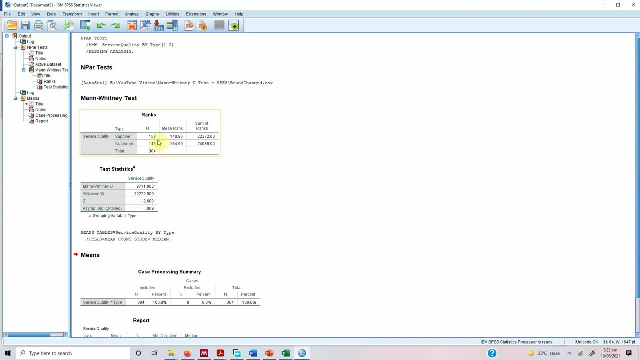 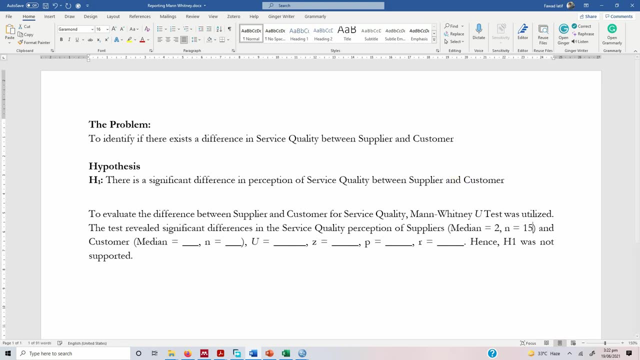 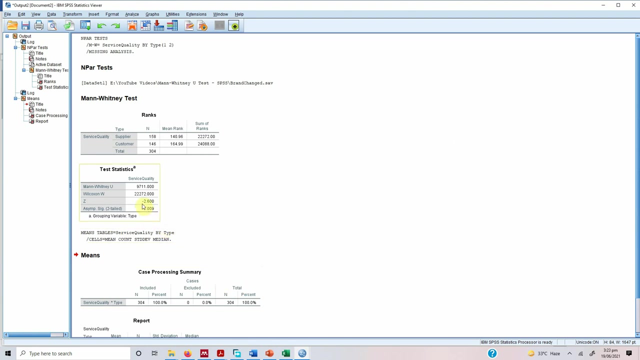 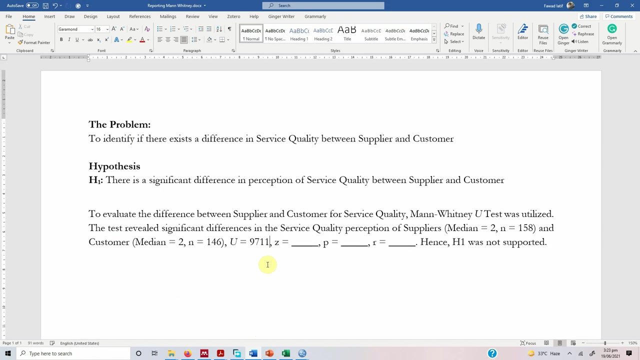 is 158 and 146 respectively. 158 and this is 146. the median value for both the groups is 2.. The U value is- here we look at it- 9711.. The Z statistic is 0.14, 0.14..